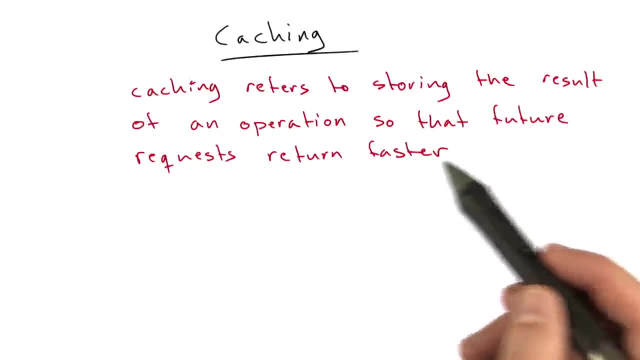 Caching refers to storing the result of an operation so that future requests return faster. Basically, if you do something once- whether it's a database query or rendering some HTML or anything that might be slow- you store the results so you don't have to do the computation a second time. 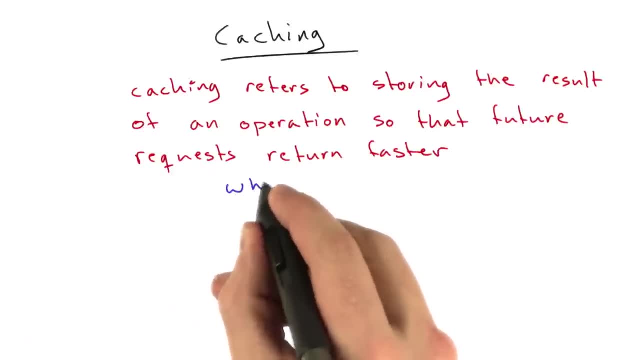 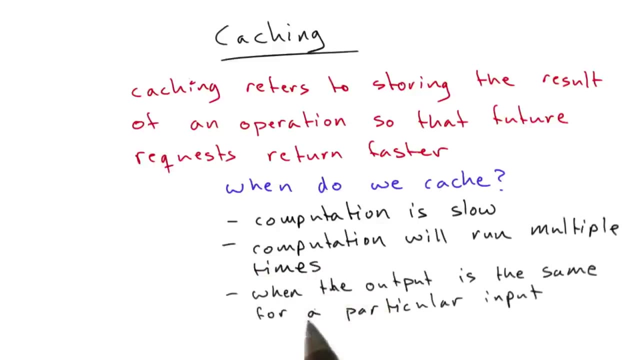 Instead, you can just reference the previous result. When do we cache? We cache things when the underlying computation is slow, when the underlying computation will run multiple times, when the output of said computation is the same for a particular input, so that we know we don't have to recompute it every time. 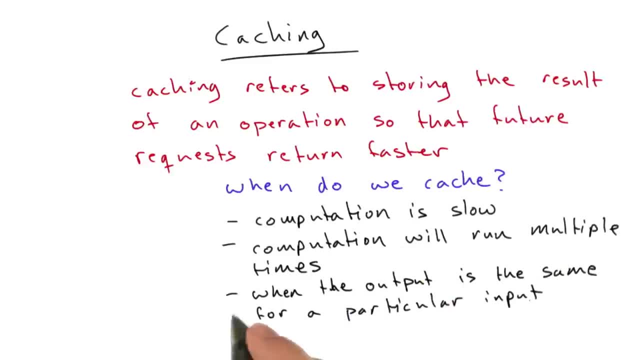 because it's going to be the same every time: the output of this computation. Another good reason for when we cache is when your hosting provider charges for DB access, which applies to you right now. Google App Engine gives you a fixed number of reads and writes to the data store in a particular day. 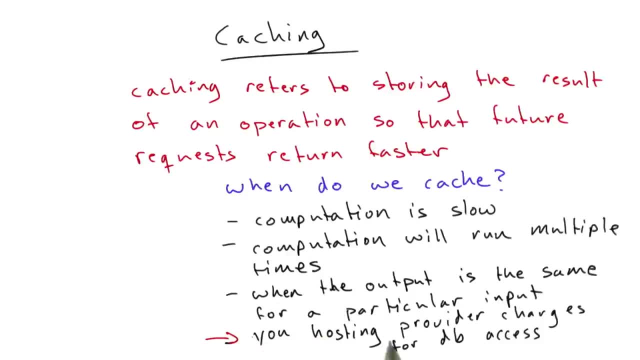 and if you go over that you have to pay for it, Even if your website doesn't get a whole lot of traffic. caching requests- so they don't have to hit the database over and over- is a fine way to save some money, and that will be an example we start with shortly. 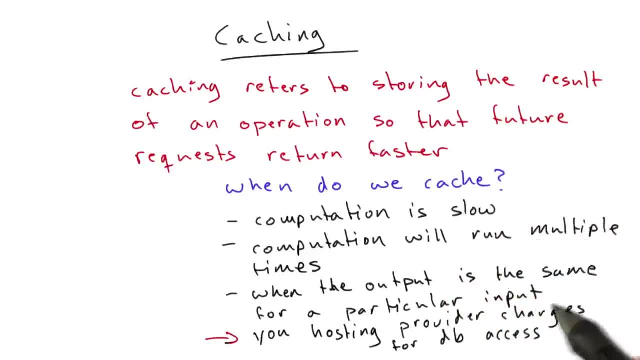 Whenever you have a situation where you have the slow computation that you're running multiple times with the same output over and over, you should cache it. You should store that result somewhere else so that you don't have to run that computation over and over. 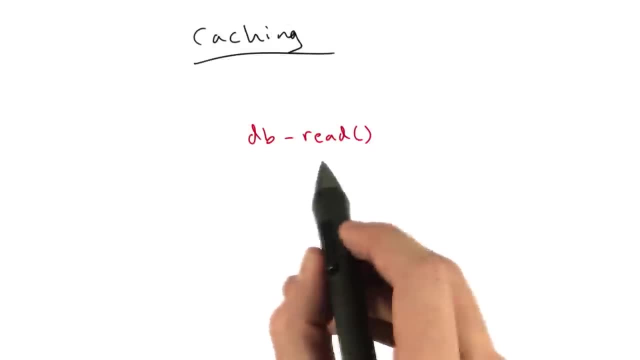 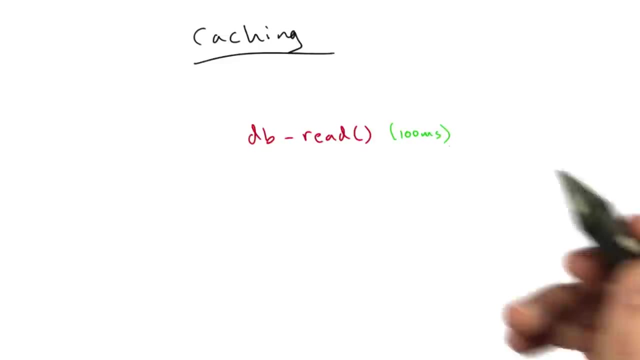 Let's talk about how that algorithm looks. Let's say we have a function called dbread and this reads from the database and it's slow. Let's say it takes 100 milliseconds to run. This is slow for a database query, but not unheard of. and you're serving thousands of requests. If every request that comes in to your website has to hit dbread, and that takes 100 milliseconds, that means you can only do 10 requests a second, or you start doing multiple requests at the same time. 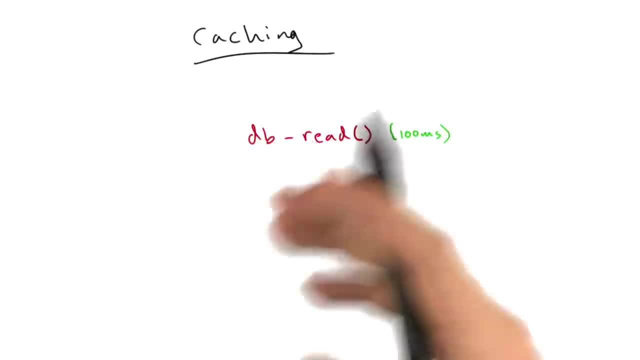 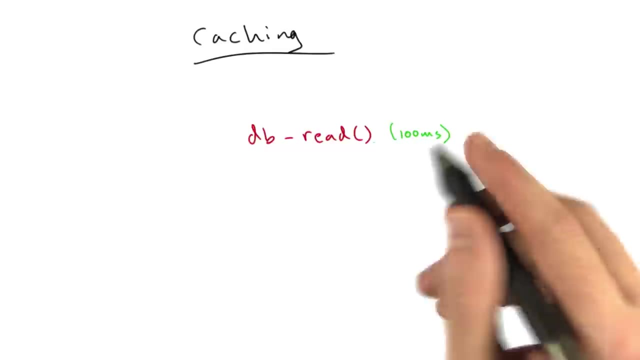 and your database starts to get pummeled because it's trying to do this complicated query all at the same time and this 100 milliseconds maybe turns into 200 or 300 milliseconds or 500 milliseconds, Who knows. When your database is under load, it starts to really get angry at you. 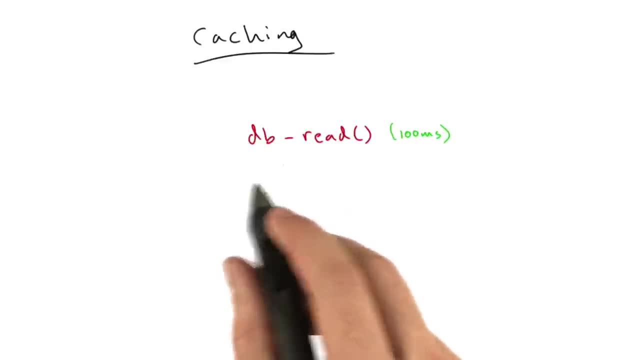 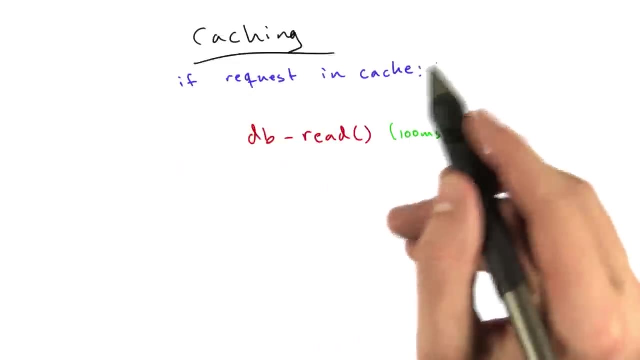 If we wanted to cache this dbread, let's talk about what this algorithm would look like. If we were to write in pseudocode here, we would have something that looks like this: If the request we're making is in the cache, return the cache version of that request. 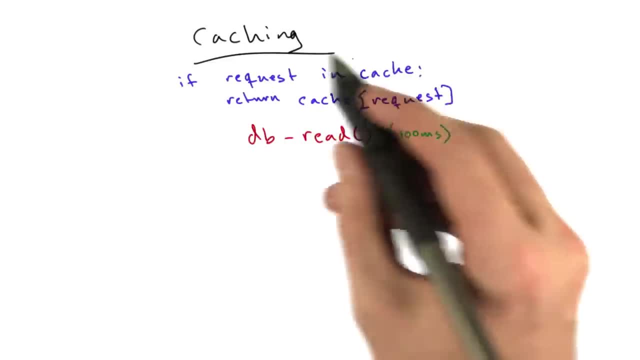 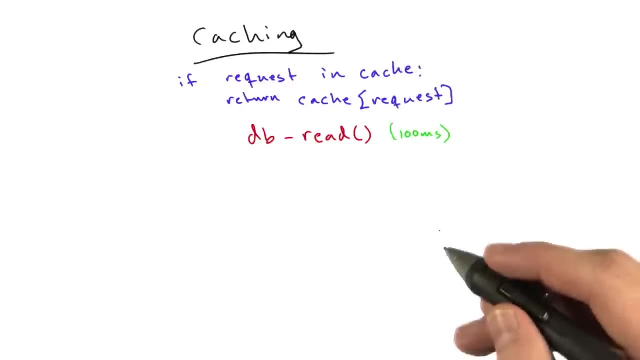 In this case I'm pretending. cache is like a dictionary and the request that we're making is a key into this dictionary. That's generally the structure of a cache. A cache is basically like a large hash table, a large mapping of keys to values. 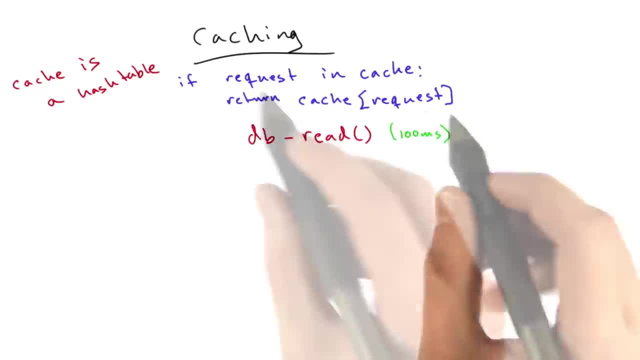 You know all about hash tables. A hash table works perfectly well. If our request is in the cache, return the cache value of that request, Else store the value of this dbread in a variable. put that variable in the cache for future lookups. 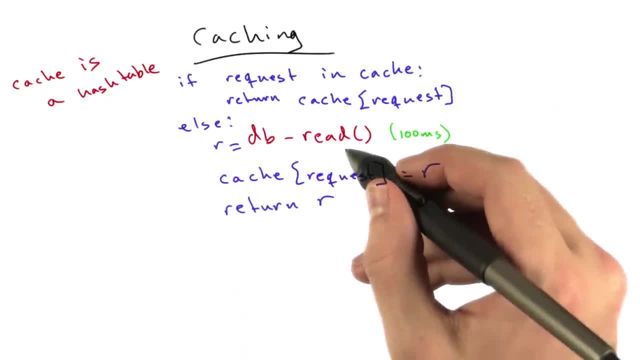 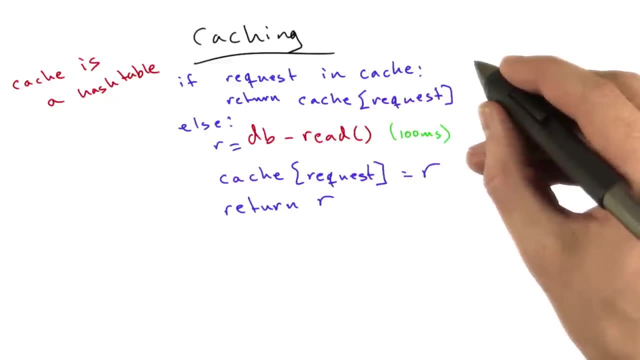 and then return that variable. Basically, instead of calling dbread on every request. the first thing we do is check to see if that request is in our cache. If it is, we return the cache value. This is called a cache hit. 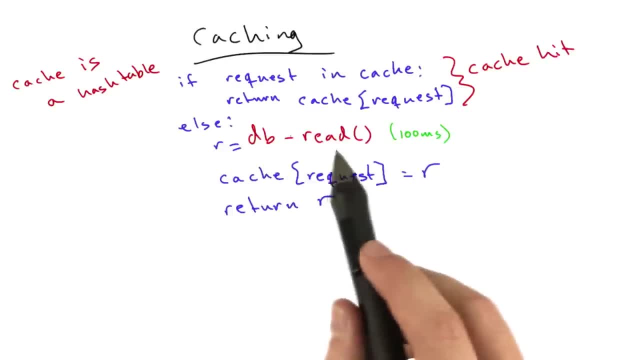 Only if that request isn't in our cache do we actually run our query. This is called a cache miss. What we do on a cache miss is we actually do our operation and store the result of that operation in our cache and then return that result. 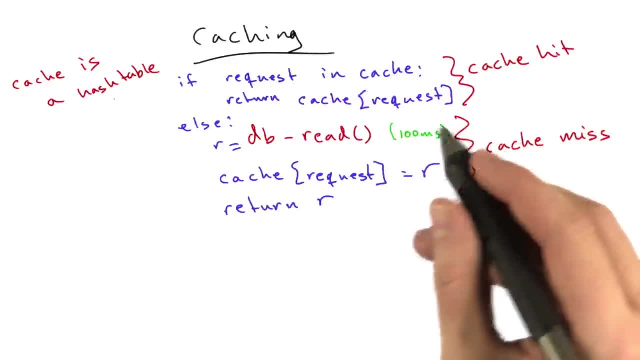 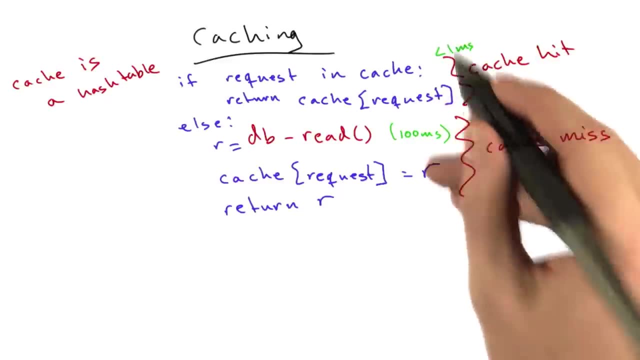 Future requests will just bounce off the cache. If you're using a hash table, depending on the size of that hash table, we're going to probably do a lot better than 100 milliseconds. We're probably going to be talking about less than 1 millisecond. 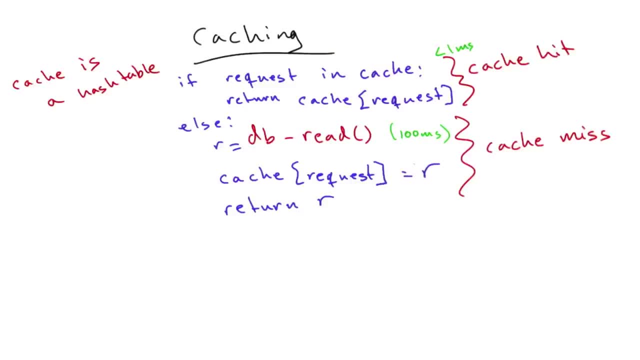 which would be quite a big speed improvement. Of course, if this hash table is huge and you're caching lots of things, hash tables have their own performance characteristics that you'll have to take into account, but you can get substantial improvements just by taking the slow pieces of your code. 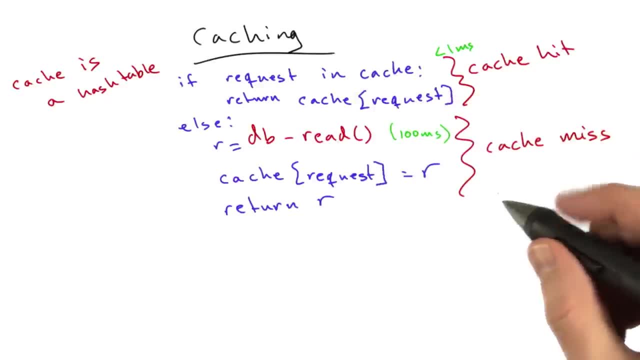 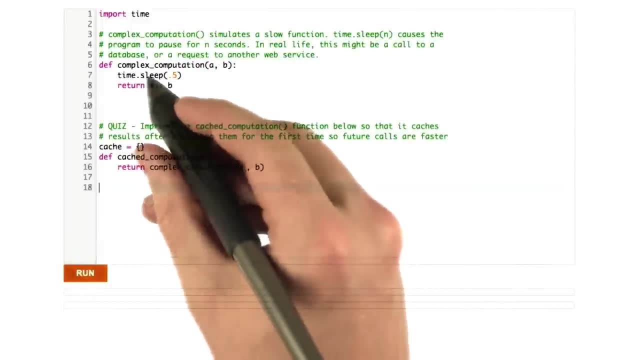 and wrapping this simple algorithm around it, which is the focus of our next quiz. What I'd like you to do is implement that caching algorithm here in Python. What I've given you is a function called complex computation. This takes two numbers and it adds them up. 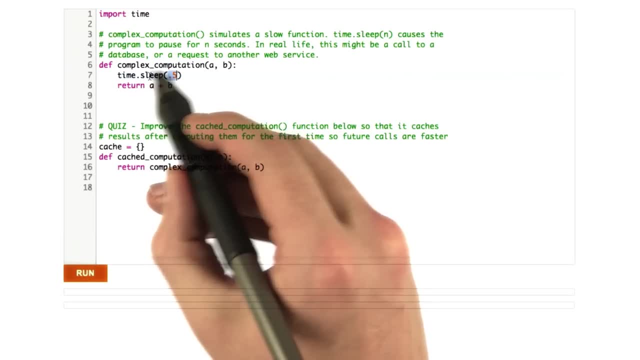 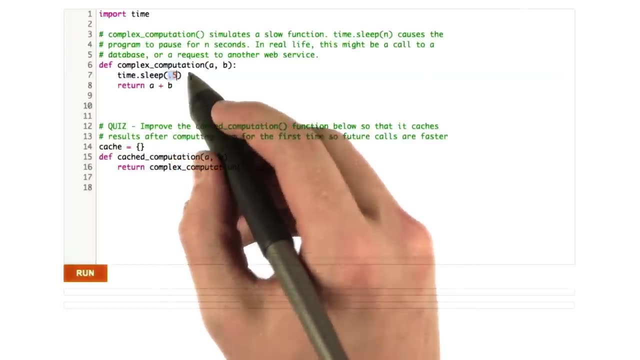 but it's going to take half a second to do so. The timesleep function causes Python to just sleep or wait for however much time you want. In this case, I have it sleep for half a second. What I want you to do is use a dictionary as a cache.